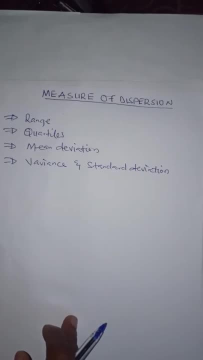 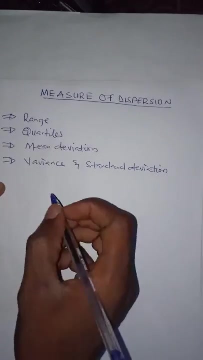 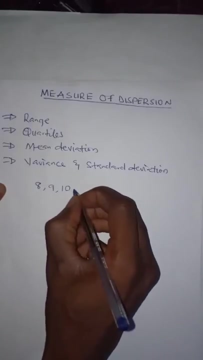 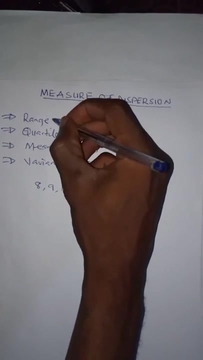 But in this tutorial I am going to restrict this discussion based on mean deviation, variance and the standard deviation. So first we have data. So first this data we have For range: range is the difference between the least value and the highest value. 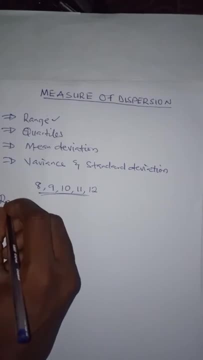 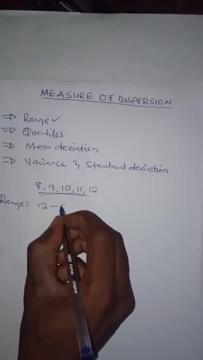 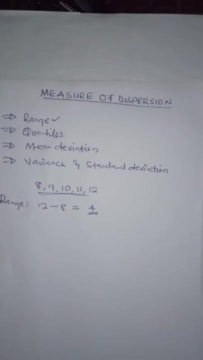 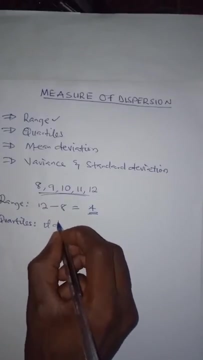 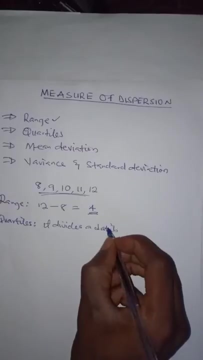 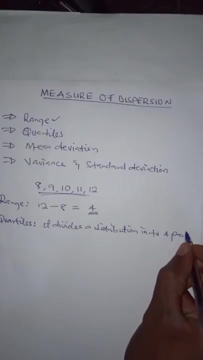 So in this set of data the range is going to be of 10 by taking the difference of 12 and 8, which is equal to 4.. So the range of this data here is 4.. What Quartiles does is this: it divides a distribution into four parts for mean deviation. 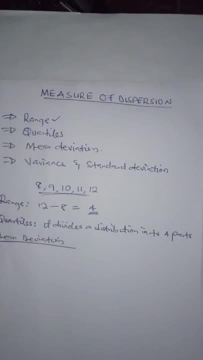 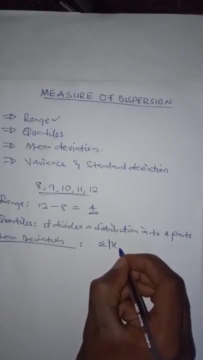 which is also very important in statistics. under a measure of this fashion, The mean deviation is an arithmetic measure. The mean of all the absolute deviation from the mean is the sum of all. the absolute deviation from the mean X bar divided by N. This is for population. 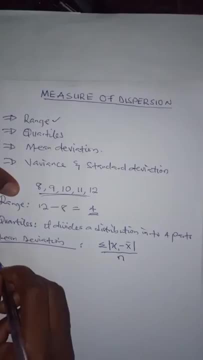 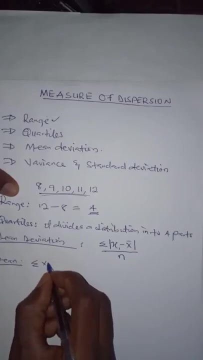 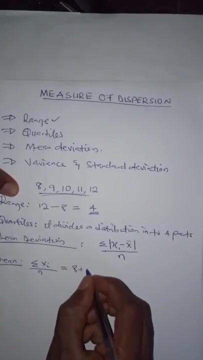 We are going to first of all find the mean of this data, which is mean which is the sum of all. So, for example, the data we have divide by the number of data, and this will be equal to 8 plus 8,, 8 plus 9, plus 10, plus 11, plus 12,. divide by 1,, 2,, 3,, 4,, 5,, all divided by. 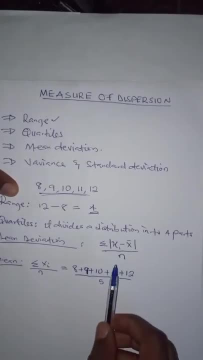 5. So if we add this together, I believe 12 plus 8 is 20.. So that's the meaning of the mean deviation. So if we add this together, I believe 12 plus 8 is 20.. 9 plus 11 is also 20, 20 plus 20 is 40 plus 10 is 50. so this is equal to 50 divided by 5, and this 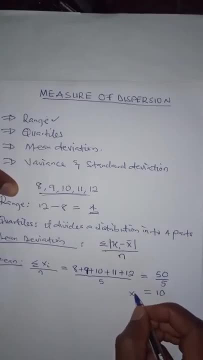 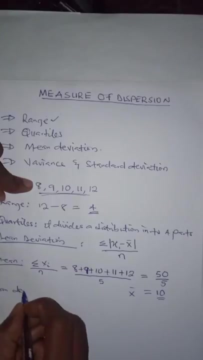 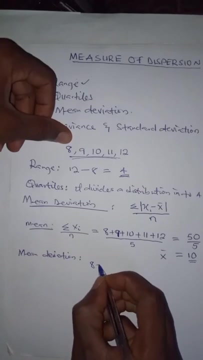 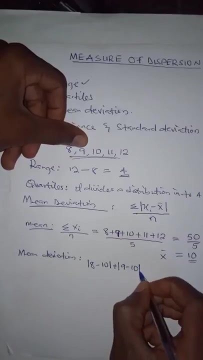 is equal to 10, so the mean X bar is equal to 10. for this distribution for mean deviation, we are going to apply this formula for on-Groove data. we see it minus the mean, which is X bar, 10. we take the absolute value, we add the second one, which is 9 minus 10, absolute value plus. 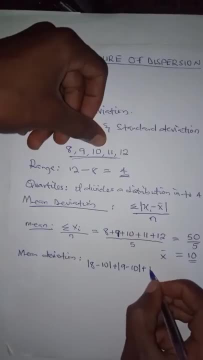 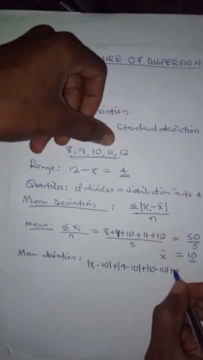 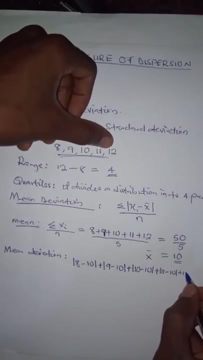 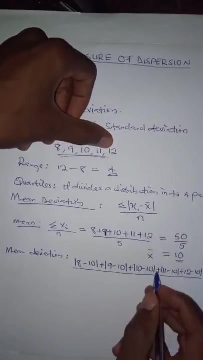 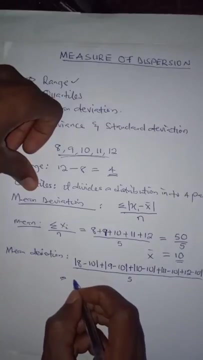 10 minus 10 in absolute form, plus 11 minus 10 in an absolute form, and the last one, which is 12 minus 10 in an absolute form, all divided by the number of times we have there, which is 5, 8 minus 10, is negative. 2 in an absolute value is going to be. 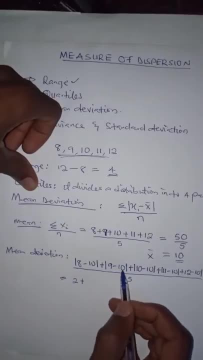 positive. 2 plus 9 minus 10 is negative 1, but in absolute form is going to be positive. 1 plus 10 minus 10 is 0. we have 0 plus 11 minus 10 is 1 plus 12 minus 10. 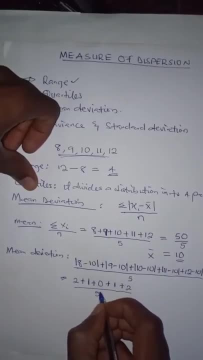 is 2. all divided by 5. 2 plus 1 is 3. 3 plus 1 is 2. all divided by 5, 2 plus 1 is 3, 3 plus 1 is 3. 3 plus 1 is 3, 3 plus 1 is 3. 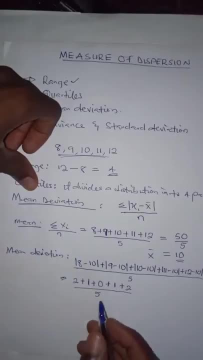 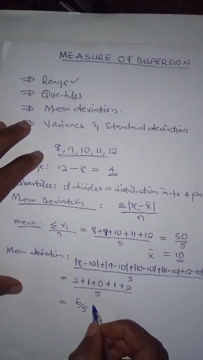 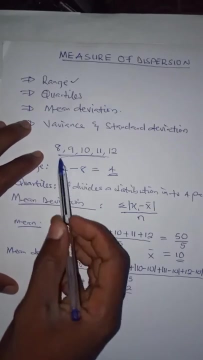 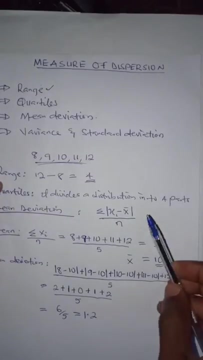 is 4, 4 plus 2 is 6, so we have 6 over 5, which is equal to 1.2. so the mean deviation of this set of data is 1.2. but I want to talk about sample. for sample data you have to subtract 1 from n, which is going to be: 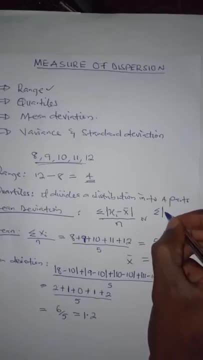 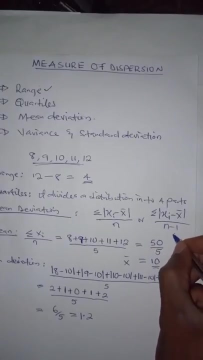 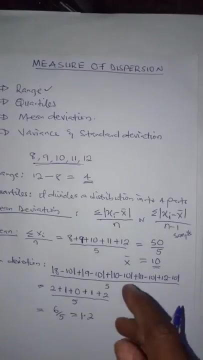 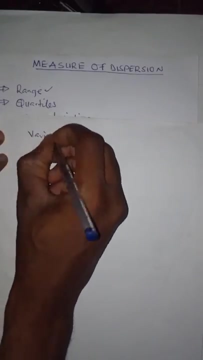 summation of the absolute form of all the data we have, minus our mean x bar, divided by n minus 1. this is for sample, sample data, which is a subset of population. so now let us look on to variance and standard deviation. for variance, there is no way you can find standard deviation without finding 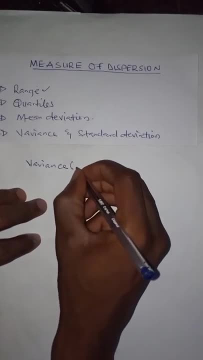 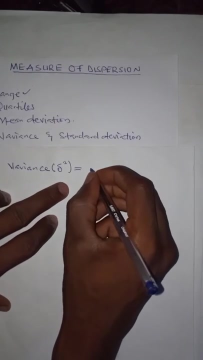 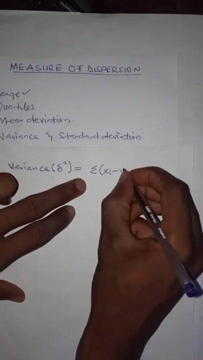 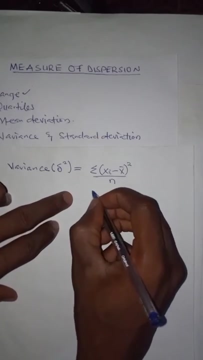 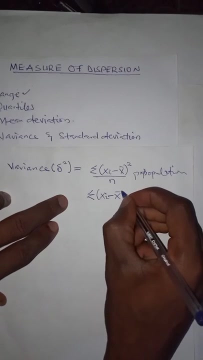 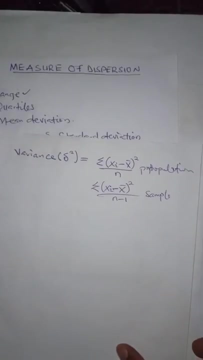 variance. so variance which is denoted as Sigma square, is equal to the summation of X minus X bar squared all over n for a population guards, an applying or X. this is for population- or X minus X bar squared over n minus 1 for sample variance. so, considering this data we have initially, this is the data we have. 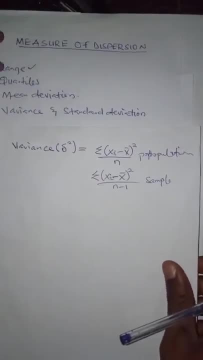 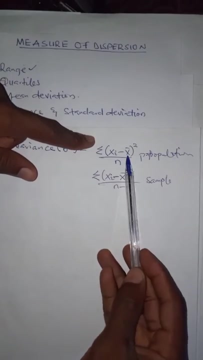 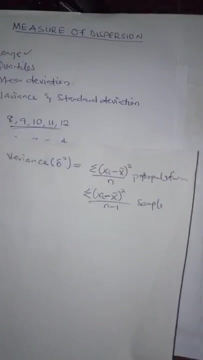 8, 9, 10, 11, 12. so to find variance of that data we are going to take each of those times, we subtract the mean, then we square, we take the summation of all. so the first one we have is 8. we have 8 minus 10, which is the mean. then we. 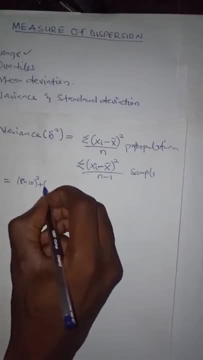 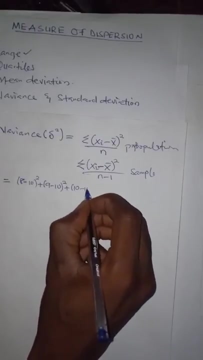 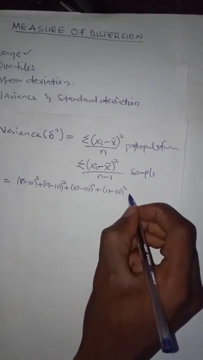 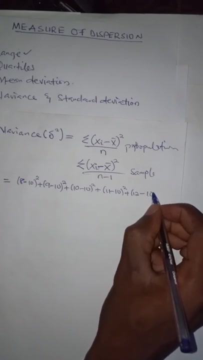 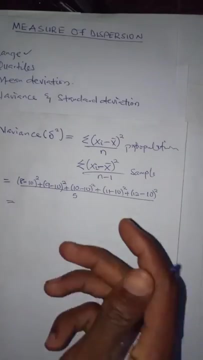 square the terms we add. the second term is 9 minus the mean squared plus 10 minus 10 squared. 11 minus 10 squared plus the last time, which is 12 minus 10 squared. all divided by number of times, which is 5, this is equal to negative. 2 squared is positive. 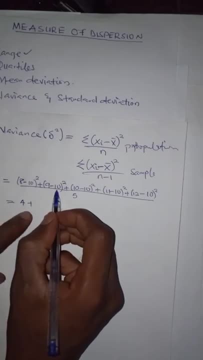 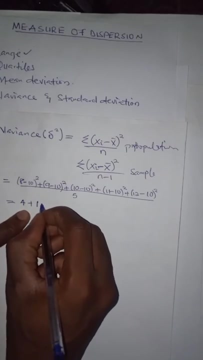 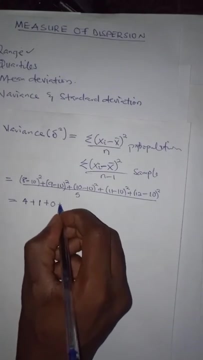 4 plus 9 minus 10 is 1. squared is 1. 9 minus 10 is negative. 1 squared is positive. 1 plus 10 minus 10 is 0. squared is 0. 11 minus 10 is 1. squared is 1. 12 minus 10 is. 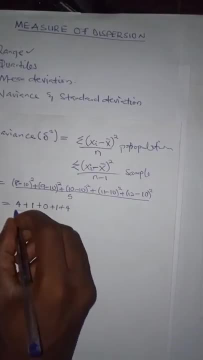 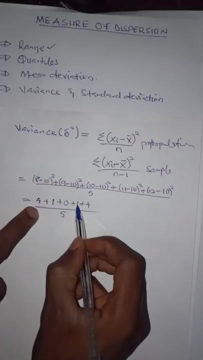 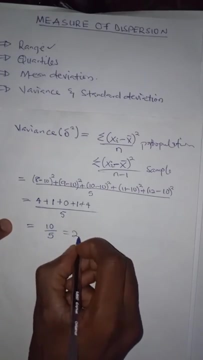 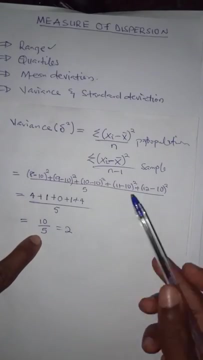 2 squared is 4 divided by 5. 4 plus 1 is 5 plus 1 is 6 plus 4 is 10. so we have 10 over 5, which is equal to 2. so the variance of this set of data is 2. this is for population variance and for sample. 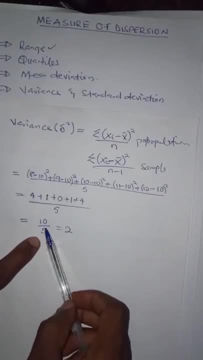 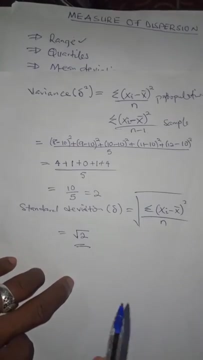 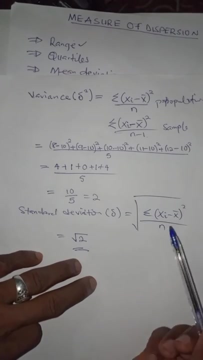 variance, you have to subtract one from the n, which in this case we will have 4. 10 divided by 4 will be our sample variance. so for standard deviation, I told you standard deviation is just the square root of variance. so this is the formula for variance we have. so we are going to take the square root of variance. 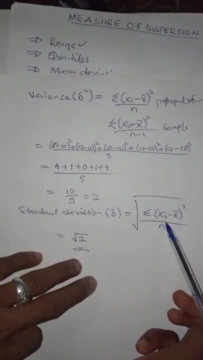 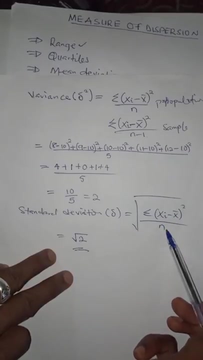 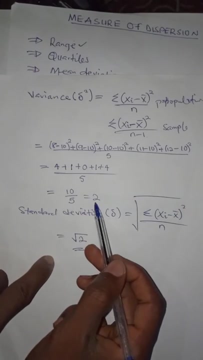 so we are going to take the square root of variance, which is the square root of the summation of x minus x bar squared over n, and this is for population standard deviation. for sample standard deviation, we are going to take the summation of x minus x bar squared all divided by n minus 1. so since our variance is 2, our standard deviation 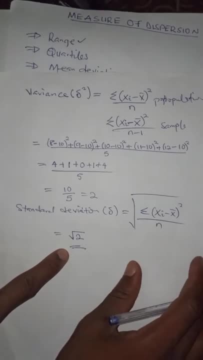 is going to be square root of 2, so this is all i have for you today. thank you for watching. do have a nice day. 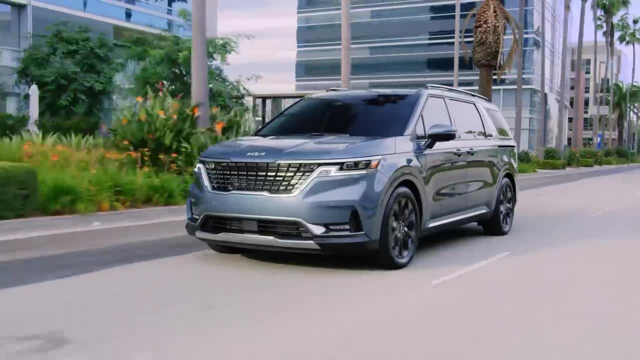 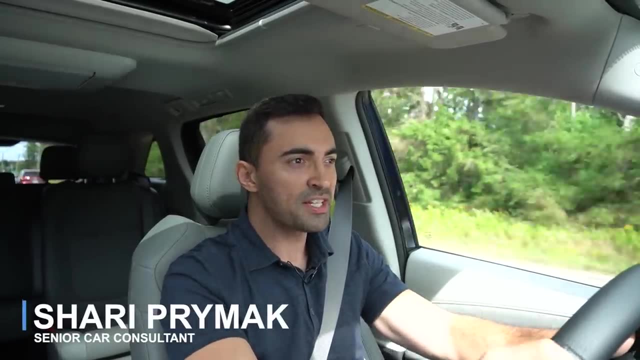 2023? Toyota Sienna, Honda Odyssey and Kia Carnival. Which is the best minivan to buy? That's what we're going to find out. Welcome to Club Corner, where we help you, the consumer, master the process of car buying and car ownership, Even though minivans are nowhere. 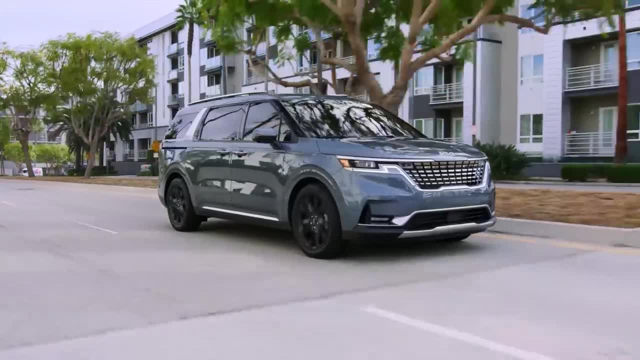 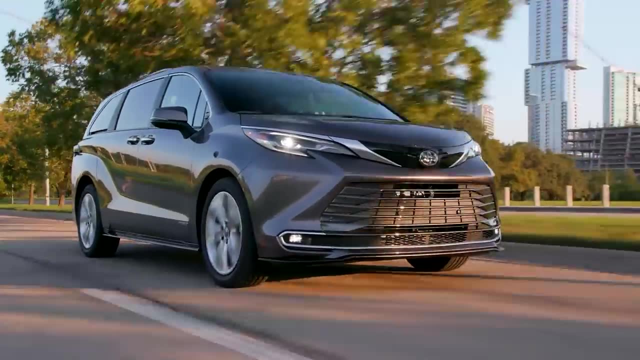 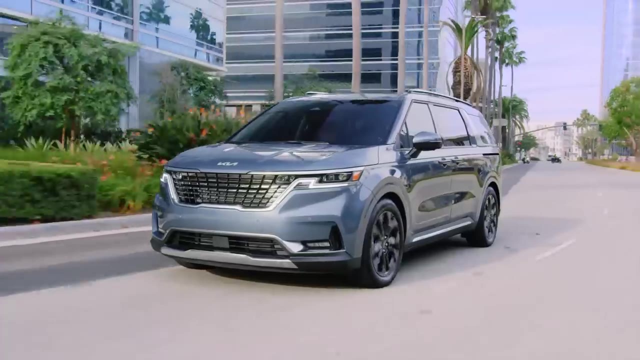 near as popular as crossover SUVs, they are still the superior choice for those who prioritize practicality and having the most amount of interior space possible. A few of the only remaining options that are still available on the market include the Toyota Sienna, the Honda Odyssey and the Kia Carnival. You could also consider the Chrysler Pacifica. 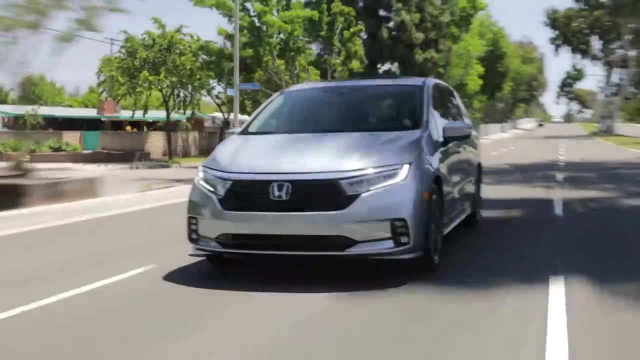 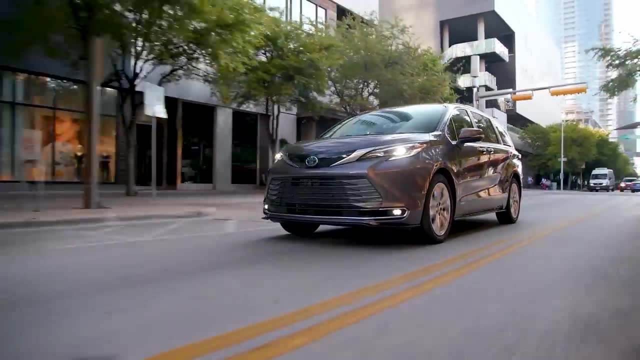 but I'll touch on that one towards the end of the video. So how exactly do these three minivans compare in terms of their performance, safety and technology? Which one has the best reliability and offers the best value for your money? Well, make sure to stick around until the end of the